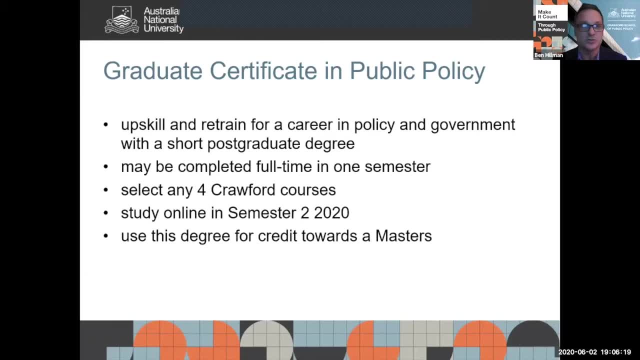 taking on this challenge in semester two and you'd like to take on a master's degree and do it full-time. you'll be able to do the Graduate Certificate fully online because I think, as most of you are aware, all of ANU's courses in semester two will be available in 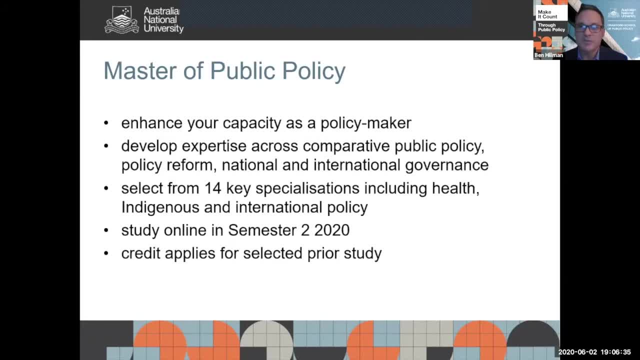 fully online mode. The Master of Public Policy is the two-year master's degree and it's designed for people who want to start or advance their careers in the public sector, with a particular focus on policy analysis. Our graduates can be found working across federal and state government agencies, NGOs. 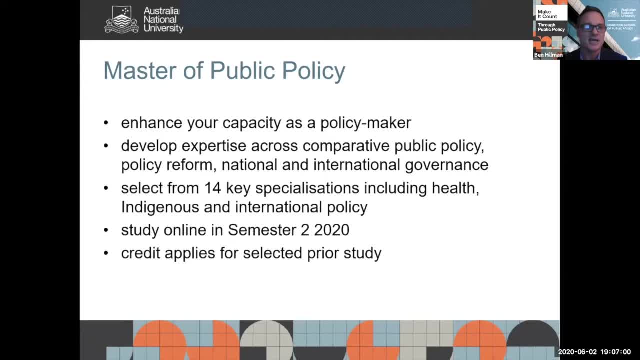 advocacy groups and in various UN and international bodies. The degree offers a wide range of specialisations in different policy areas, enabling you to really sink your teeth into sectors that are of interest to you or sectors that you'd like to build your career in, And it is possible to graduate with a Master of Public Policy, but it's also possible to graduate with a Master of Public Policy. and it's also possible to graduate with a Master of Public Policy. and it's also possible to graduate with a Master of Public Policy. and it's also possible to graduate. 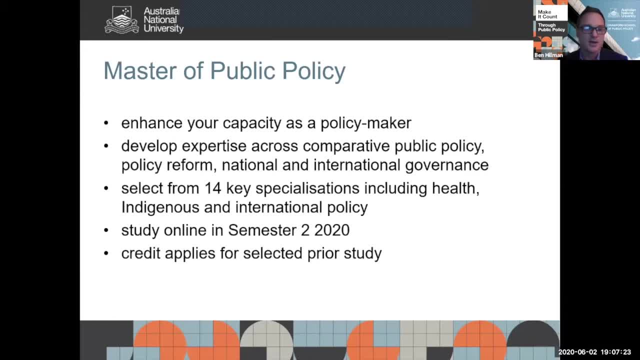 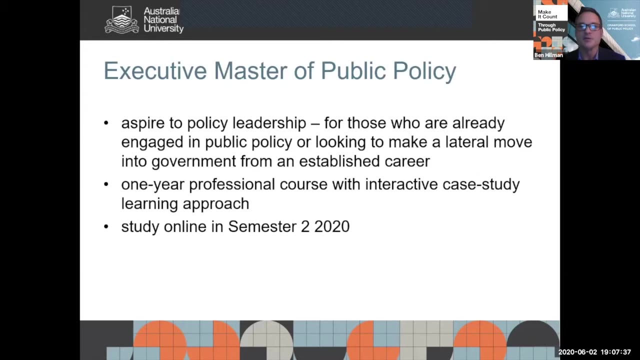 two specialisations. Graduates with relevant backgrounds can earn up to a year's worth of credits for past studies. The Executive Master of Public Policy, for those of you with the appropriate backgrounds, is a one-year program designed for emerging public sector leaders. So to be admitted. 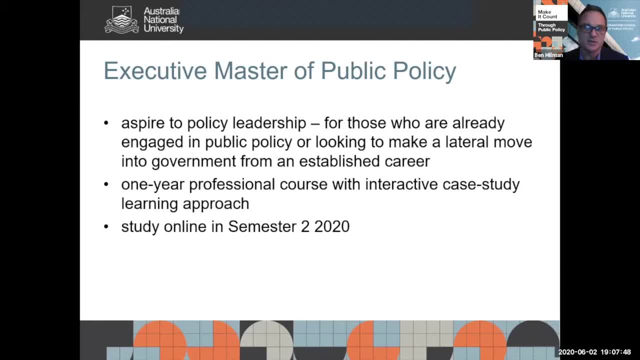 to this degree you need at least seven years of relevant experience in the public sector, in government or in other public sector agencies. It's an interactive program that draws from a lot of case-based teaching and on participants' own experience. For those of you. 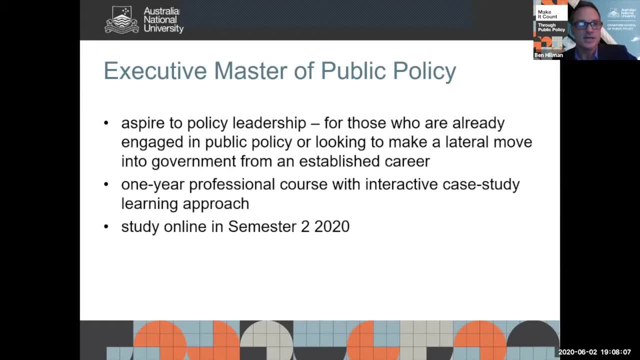 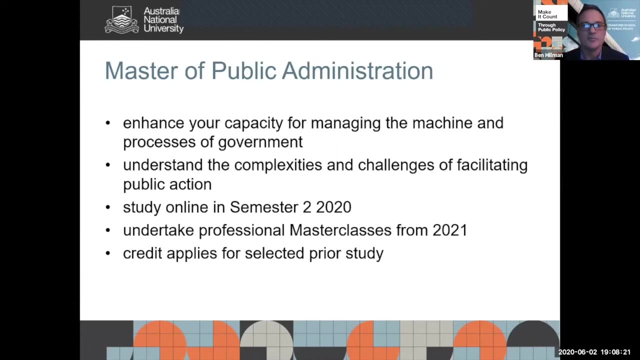 who are interested. I'm very happy to field inquiries later. It's not updated and the information is not available on the website yet, but from 2021, this degree will be available fully online: The Master of Public Administration. I'm very excited to announce 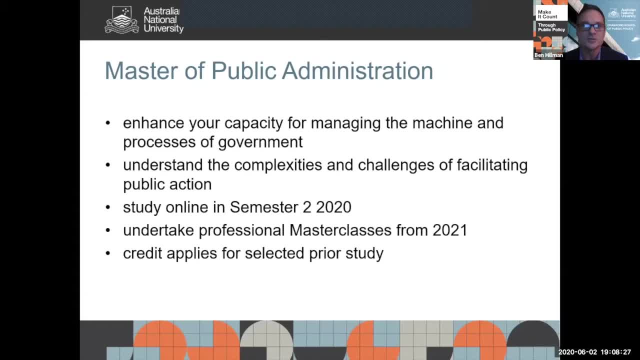 is a degree that will be relaunched in 2021.. It's a brand new one and a half Master of Public Administration that's designed for public sector managers, And this is perhaps the main point of distinction between the MPA and the MPP. The MPA is more focused on 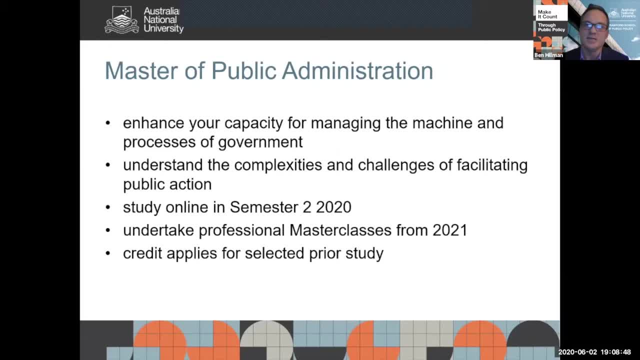 management and the MPP tends to focus more on analysis, But in reality, of course, both at senior levels of public sector agencies, both skills are, of course, both capacities are really important and there is a lot of cross-fertilization across the degrees in the electives that. 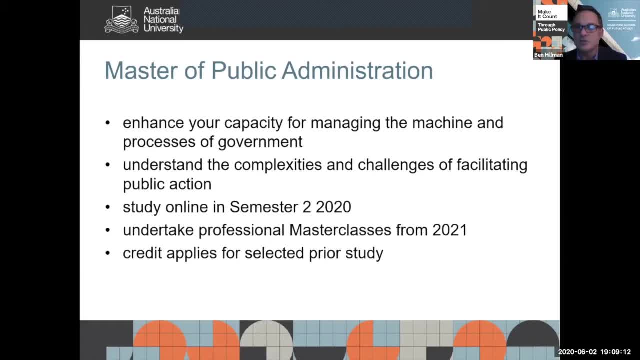 you're able to take The MPA. the new MPA introduces a series of applied masterclasses in leadership, strategy and financial management, And this is an opportunity to get skills and learn from practitioners as well as academics- people who are really at the. 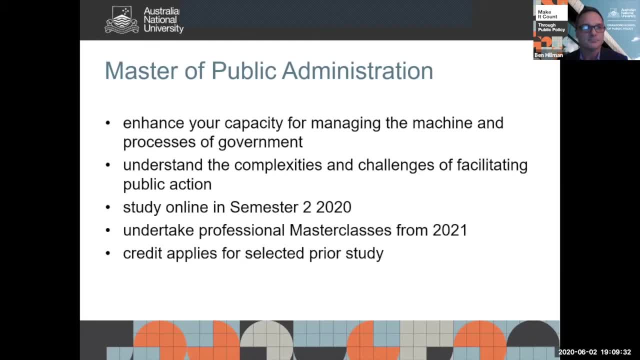 coalface of management and policymaking. Students will also complete the MPA with a capstone project, either an internship for people doing the degree full-time and with limited professional experience, or as a practice-based, work-based project for those who are already employed in the public. 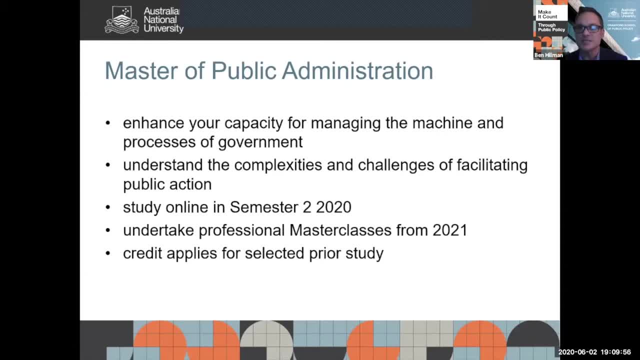 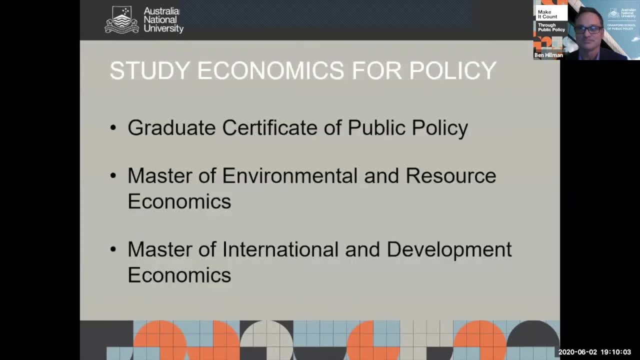 sector. So that's it. That's a snapshot of our four degrees, and look forward to fielding questions that anyone has later on. Le Gan Yuyang. Oh, there you go, you're on. Okay. Yeah, Hello everyone, My name is Le Gan Tsung. I'm the head of 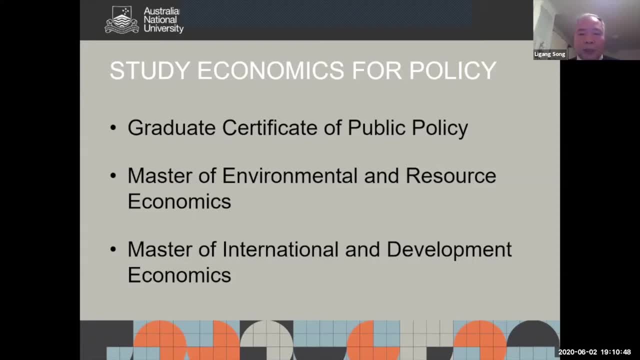 the department of economics. The department is uniquely positioned in the College of Asia Pacific and, as you know, later on we have a, you know, wider range of country and area studies. The department also uniquely positioned in the public policy school. so therefore, you know we have a very strong policy orientation in terms of our teaching. So, basically, our principles of 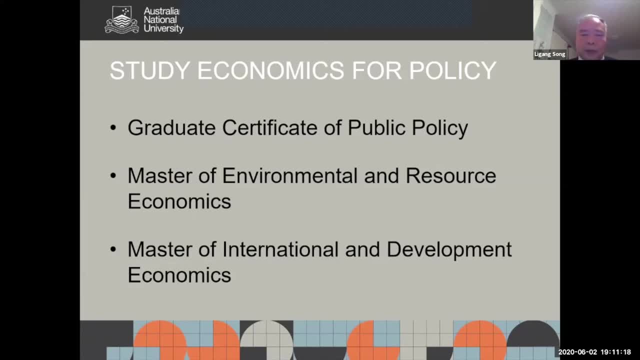 for offering those degrees. number one is about a very solid theoretical underpinnings. The second one is about you know the policy, actual policy studies. The third one is that we equip you with a very stringent and rigorous quantitative methodology and skills, And with that one. so let me just go through with you about the three things. 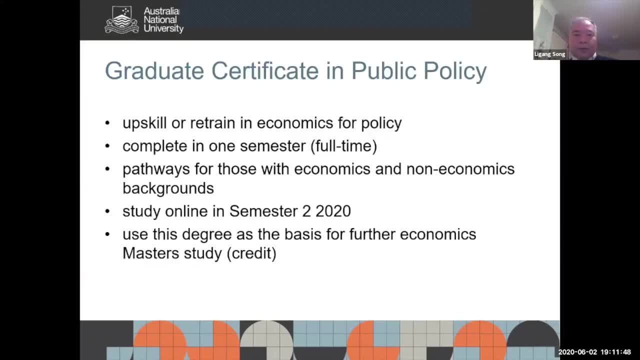 Number one is: we want to page next one. yeah, so this. I see this is the, I think, mentioned that one in the sense. no so, graduate certificate in public policy. So in this area we are, you know, it's kind of a certificate, you do, it's not a full. 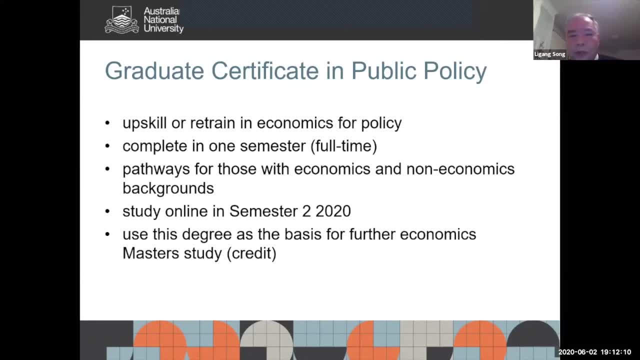 degree courses, but you do up to three or four courses for doing that one. Most importantly, you know in the sense, is the is to give you some kind of retraining in economics for policy discussion and and, and and and understanding the policy debate, and you can complete this certificate. 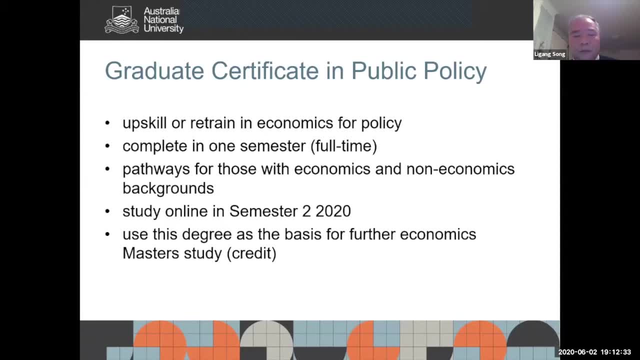 in within one semester. Of course you have to do it as a full time and by doing so that can give you the the pathways for those with economics and the non-economics background, Meaning the pathway you do a bit of a full degree later on. so we'll give you the necessary background for doing that one. 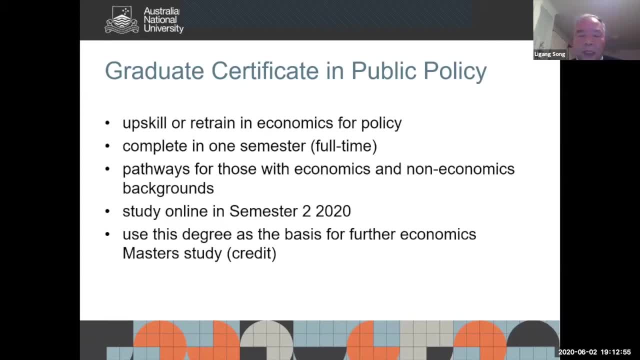 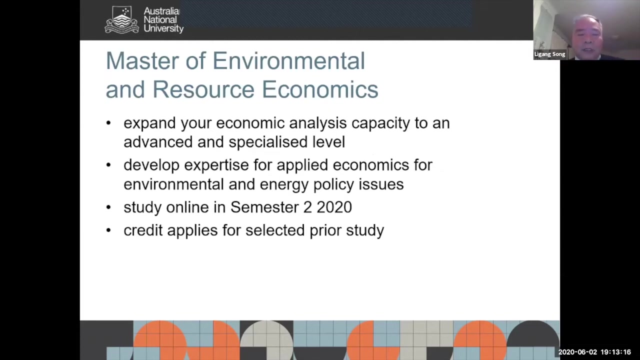 This can be offered in semester two 2020 this year, and also online. You can use this degree as the basis for further economic master studies. so that means that you take the certificate but you take the credit for doing more master degrees later on. The second one let me focus is on the 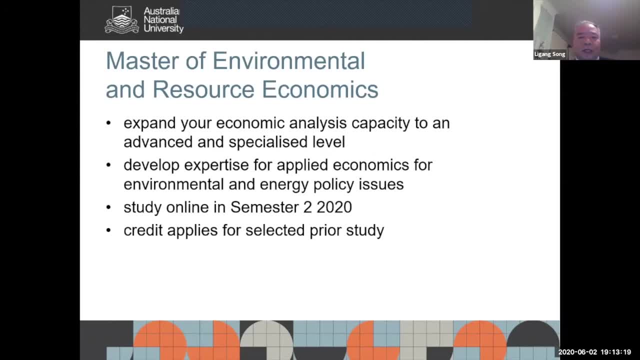 master of environmental and resource economics. So, as you can see from the title that environmental and resource economics is a very popular subject, that can expand your economic analysis. It's kind of a capacity to advance and, especially at the level, focus on the environmental and resource. 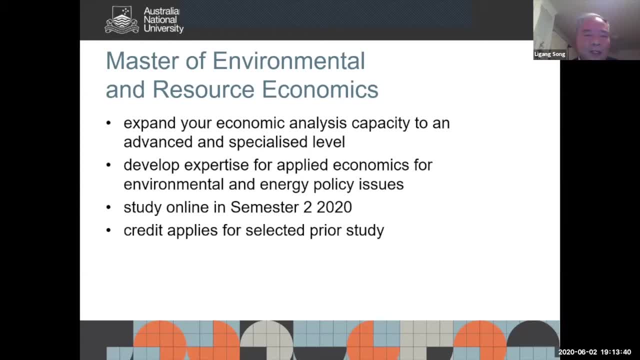 issues And subjects include water, agricultural resources and etc. So therefore you can develop the expertise for applied economics, for environmental and energy policy issues- We do have world-class scholars- and focus on those issues, and energy issues in particular- And again, study online in the semester two. Again, that is the credit you can apply. 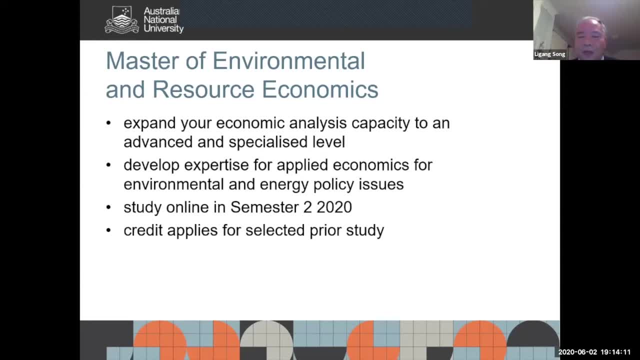 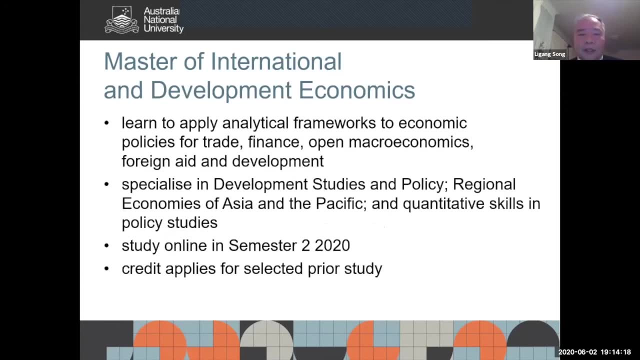 for the. I mean if you have a prior study, you know we can consider, you know, giving a credit for completing. this is a degree. The master of international and the development economic is our main degree offered through on the court and department of economics. So for doing that one, 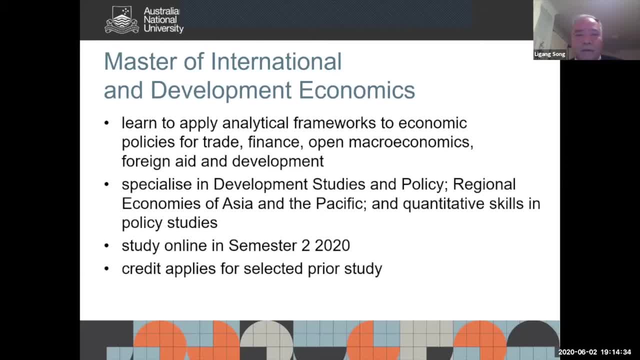 you know, as you can see from the title as a career, the focus on the international and the development economic. So we are a way to go from college in this. a lot of people is not interested in business and education to business. education is not much of an aspect but we do also have for us. 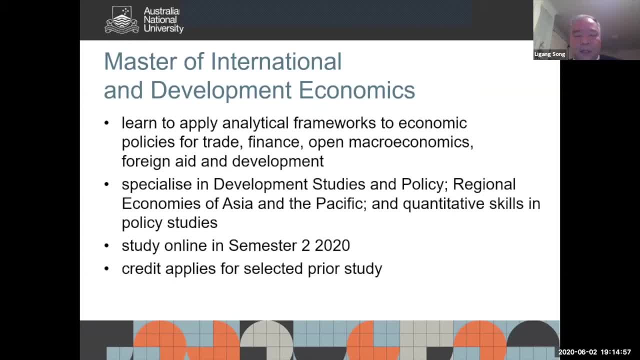 few specialization And in doing this degree you learn to apply analytical frameworks to economic policies for trade. This is a you know what's the long history of teaching trade issues in the work class, expert in teaching foreign aid and the development issues And the development again at the different levels. 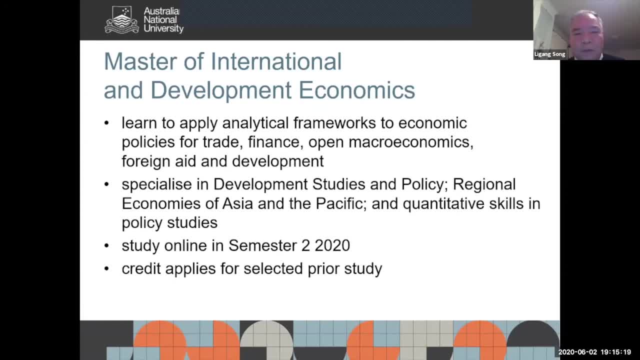 You can do this from a preliminary level to a most advanced course in economic development, And you can. as I mentioned, there's a specialization in the development studies and the policies. There's also clear focus on the regional economies of Asia and the Pacific. 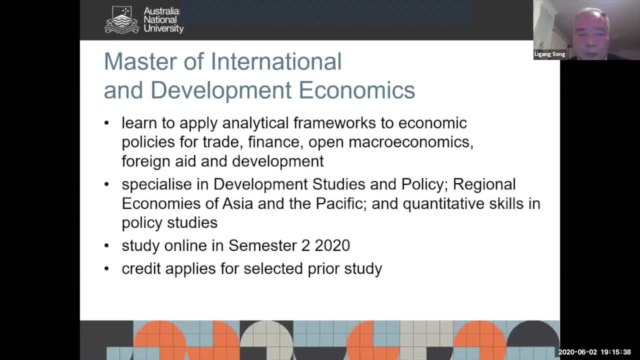 Like scholars, are specialized in Indonesia economy, the Chinese economy, the Southeast Asia economy and et cetera. The quantitative skill is also a very important part of our training. So after you got a degree, or during the training getting that degree, you will have through. 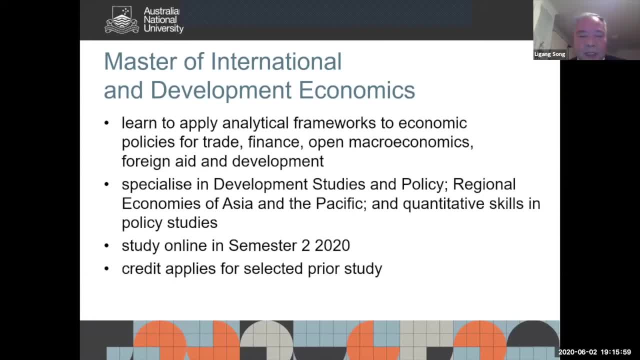 preliminary mathematical courses, but also you can get this training in the, in the econometrics and also the case study econometrics that become more and more advanced in doing so And study online in semester two this year and almost like all the courses now are being offered is online. 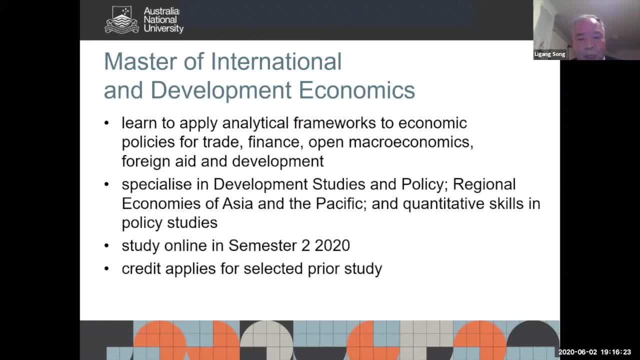 And again, if you have a prior study in the economics or the related area, we are taking into account about providing some credit for you. So all these are the degrees and in the offer and we treated the students experience in a very important way. 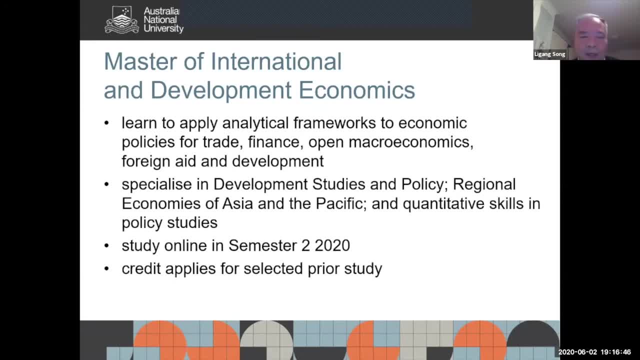 So therefore, it's not just passive learning in enrolling in those courses, but you interact with our staff in the learning process And that experience will be, I think is very valuable for you and for your study, but also for your future career development. 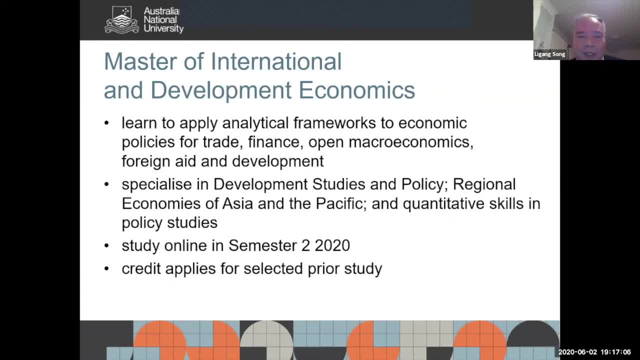 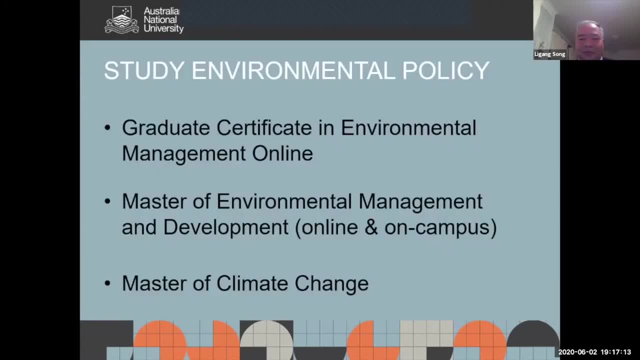 So that's a brief introduction, And I'm happy to answer your questions at a Q&A session later on. Thank you, Hi everyone. Since it's Reconciliation Week especially, I'd like to just start by acknowledging the traditional owners on whose country. 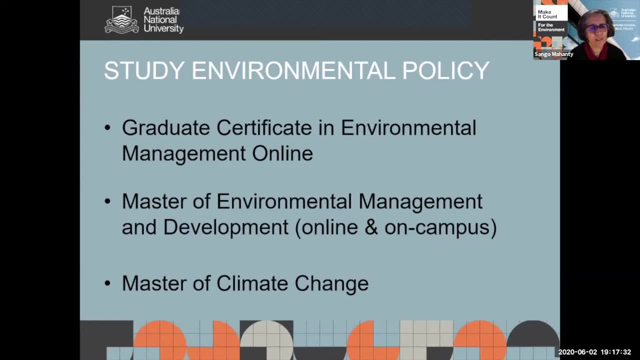 I'm speaking from today to all of you, So I'm just gonna say a few words about the first two programs that are mentioned on this slide: the Graduate Certificate in Environmental Management Online and the Master of Environmental Management and Development. So those are two programs taught from our group. 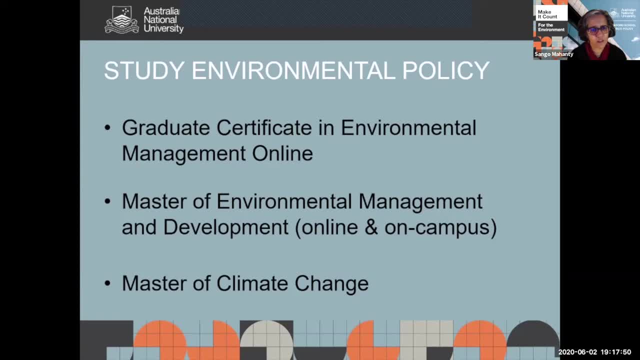 And there's a third program that we co-teach with the Fenner School of Society and Environment, which Bec will speak to after I'm through. A general comment about all of those programs is that our graduates work in all sorts of fields, quite similar to what Ben flagged, actually. 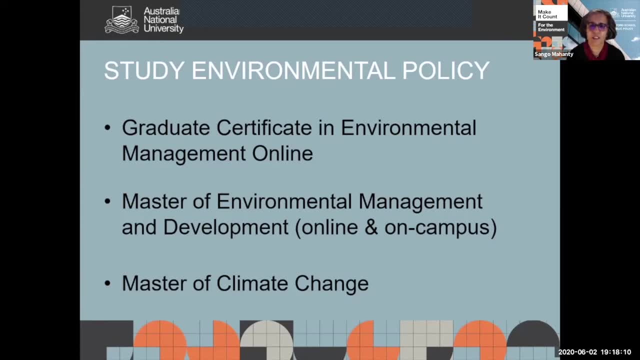 but with more of a focus on environment, specifically environment and development issues. So in government, in policy or regulatory positions, in the private sector, civil society organizations. So quite a diverse set of outcomes for our graduates. So, starting with the Graduate Certificate, 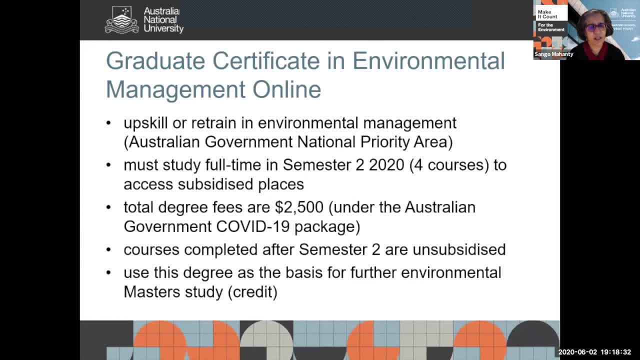 in Environmental Management Online. this is a new program that's being supported, supported by the government's higher education support package, which is available to domestic students, And it's a really it's highly subsidized. So you can see there four courses that would be undertaken in semester two, 2020.. 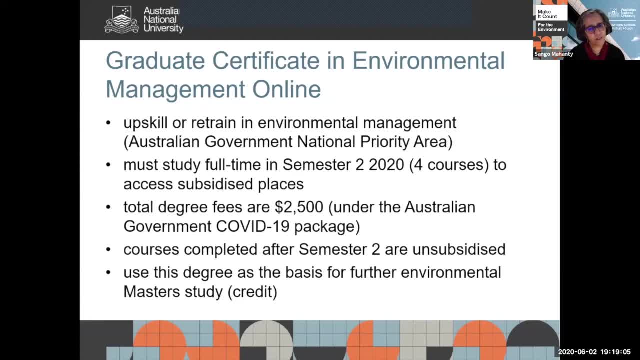 If, for some reason, a student wanted to do less than four courses and finish off the certificate in 2021,, that would be permitted, but the subsidy would no longer apply after 2020.. This is like the COVID relief package for the higher education sector. 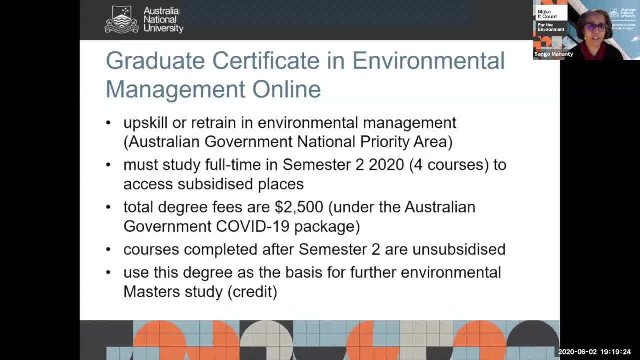 So it's for a limited time. The courses in this: we've put together a really interesting and sort of very practical set of courses. Again, we're working with the Fenner School of Society and Environment dealing with things like disaster management. 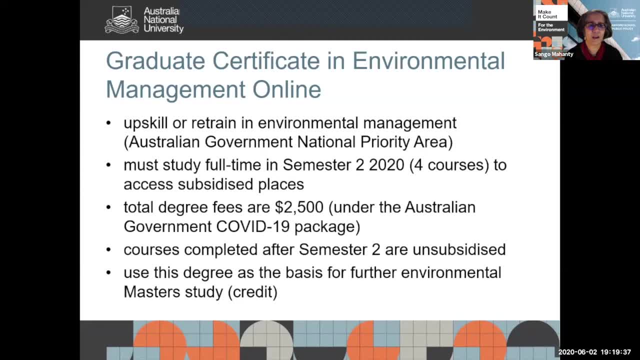 ecotourism, food security and society and environment relationships. So quite an interesting program there that's been sort of purpose built this year but actually draws on our existing offerings. And then the Master of Environmental- oh, actually similar to the, 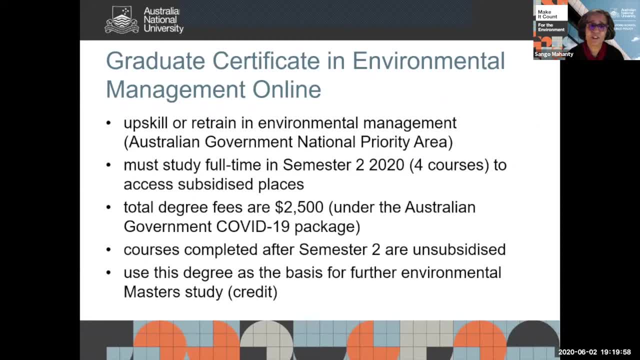 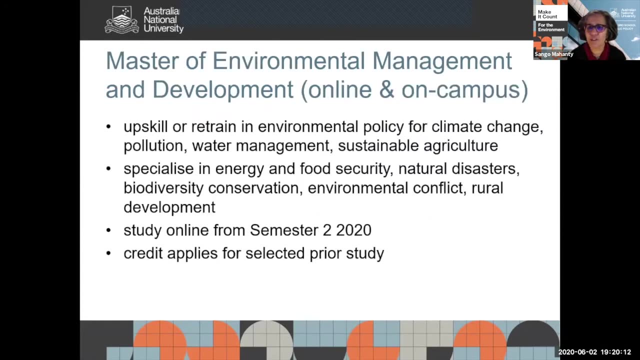 Public Policy Graduate Certificate. any courses that are undertaken in the Graduate Certificate can also count towards the Master's, if you get excited enough to carry on to some further study. So the Master of Environmental Management and Development, which I'll talk about briefly now. 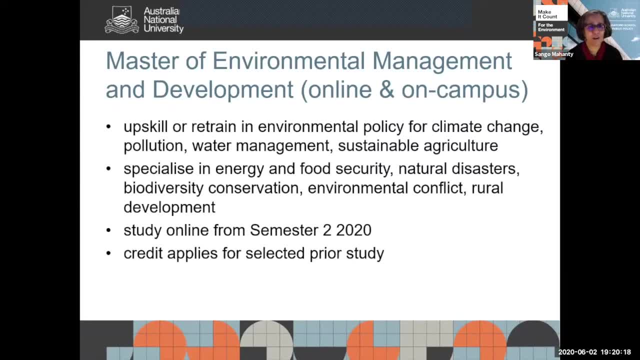 is a program that sort of broadly aims to boost the careers of people working or interested in working in natural resource management, environmental policy, in a host of different sorts of organizational settings, And it's very much about improving your professional capacity, your ability to deal with complex challenges. 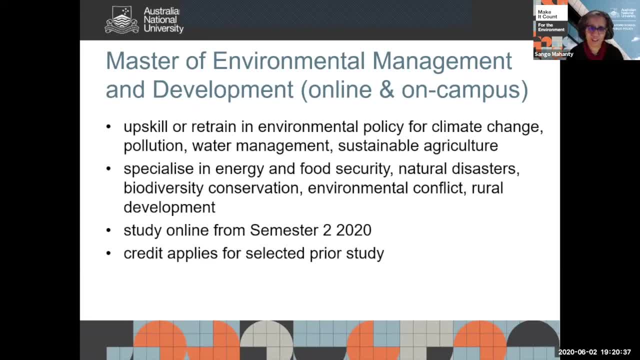 because, as we all know, working on environmental governance, environmental policy, is a very complex and multidimensional sort of process And our program is available fully online or on campus or a combination of those, So one I guess thing that sort of distinguishes our program. 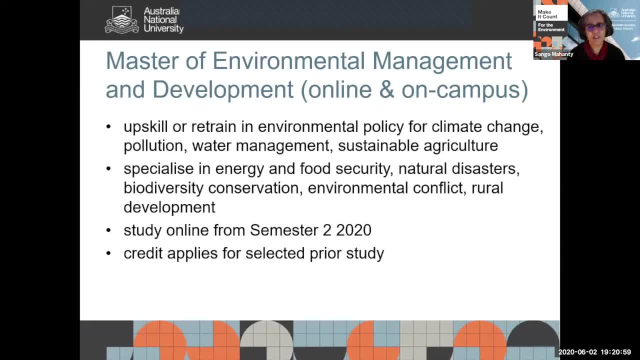 is that it's a highly interdisciplinary program. So I think this is another really interesting program, another really important way in which we think about working on environmental issues, because when I was an undergrad, one of my lecturers said to me: managing the environment is about managing people. 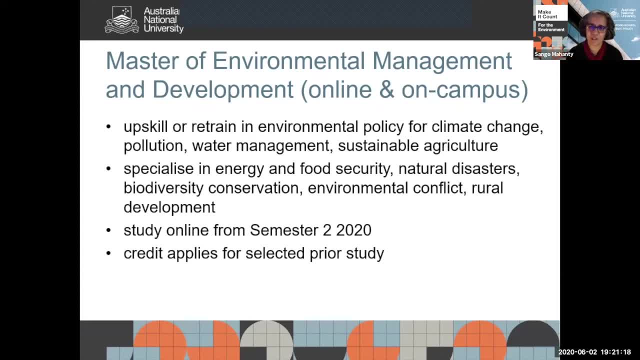 And so we really turn our attention to that side of environmental governance. We've got people in our program who are economists. I am a human geographer, we have anthropologists, So it's a very diverse set of perspectives that we think about. 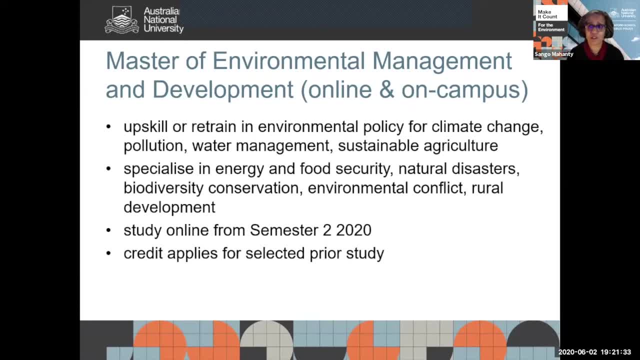 we think are quite important to equip professionals in this field and to really work on critical analysis skills, trying to understand environment from a political, social and economic dimension. And there's also electives that can be picked up that deal more with environmental science in the Fenner School. 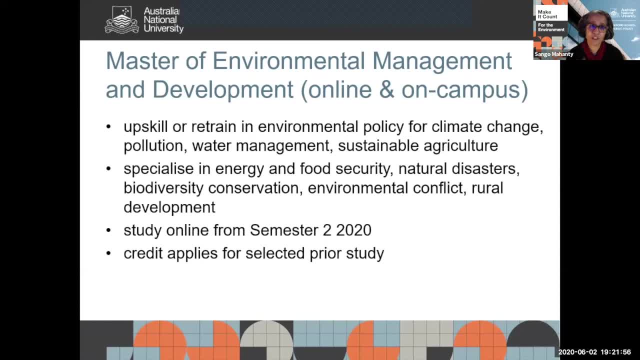 Yeah. so I guess broadly the program aims to kind of build critical thinking as well as practical skills to work on some of the really challenging issues that we're facing. So we all actively research and in areas like climate change, pollution management, we've got quite a body of expertise. 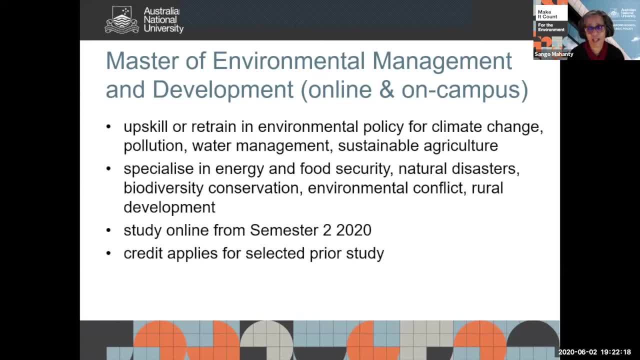 on natural resource management, things like water, forests and land, And so we bring all that into our courses and really kind of practical case examples. We like to draw that into our teaching quite a bit. Yeah, we work, our group works in Australia. 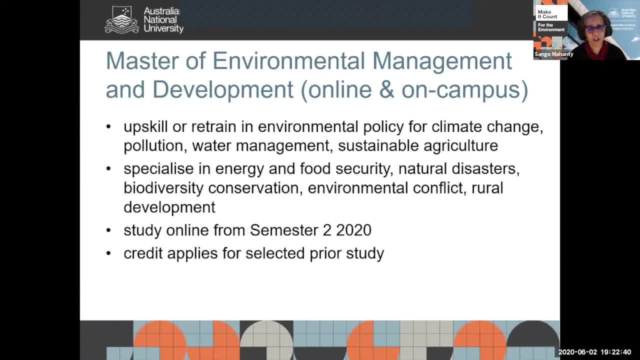 as well as in the Asia Pacific. So we can kind of move between regional and Australian case examples quite a bit in our teaching as well. So that's just a very brief overview And I might I'll just check I've covered all the points there. 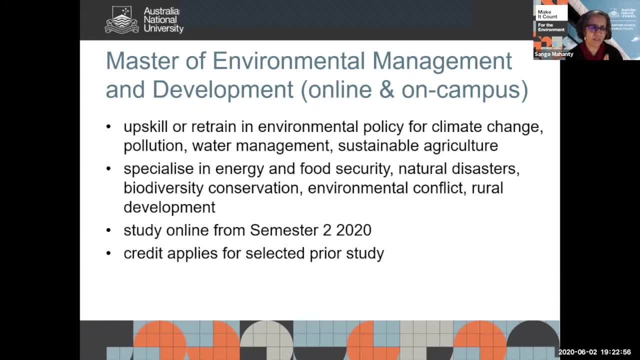 And yeah, so we the credit for prior studies- I think I touched on that- not only if you did the grad, but also we do look at kind of your past study record and often are able to sort of find areas where we can give you credit. 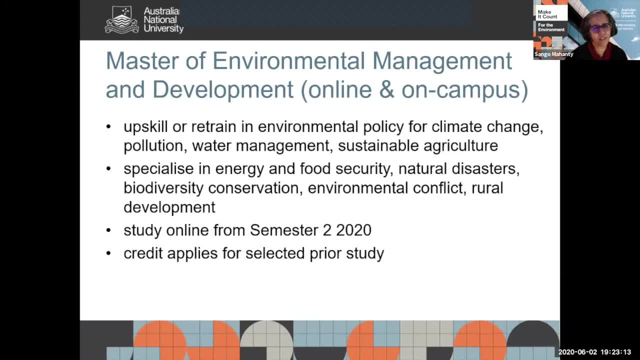 We are eventually moving to a one and a half year full-time program, but at the moment it's a 96 unit program. but yeah, we're fairly generous with credit for study in related or cognate areas. So I might hand over to Bec now. thanks. 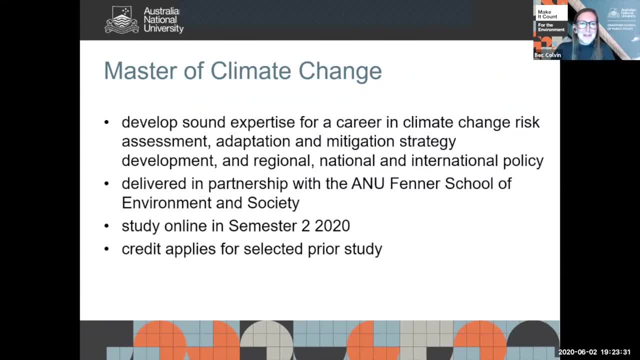 Thank you so much. Thank you, Thank you, Sango, and hi everybody. I'm piping in now because I'm an academic co-convener of the Master of Climate Change, alongside Professor Jamie Pittock at the Fenner School. 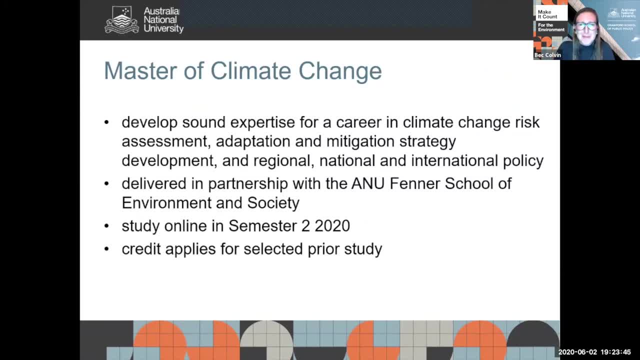 So the Master of Climate Change is a really cool program. It's multidisciplinary, as it must be if we're dealing with a complex issue like climate change, And in taking the Master of Climate Change, you go over some foundational concepts that cover environment and society. 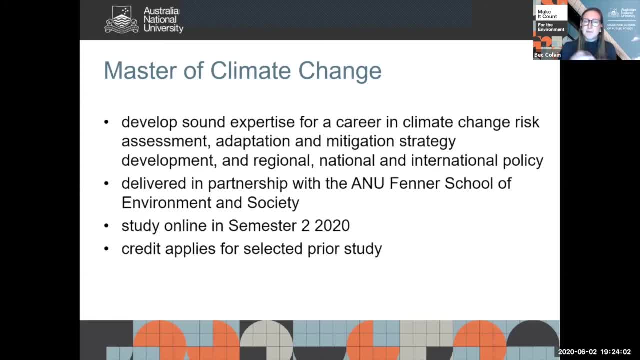 interactions, as well as environmental science, And then you move into the core climate change courses. So this is where you'll study international climate change policy and economics, domestic Australian climate change policy and economics, adaptation, vulnerability, impacts of climate change and climate science. 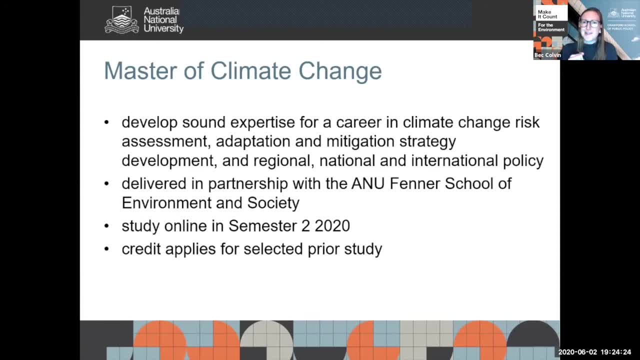 You'll also do an independent research project, So we try to get you to do this at the end of the program, as it's a place where you can Really integrate all of the things that you learn and synthesize it and build your new contribution. 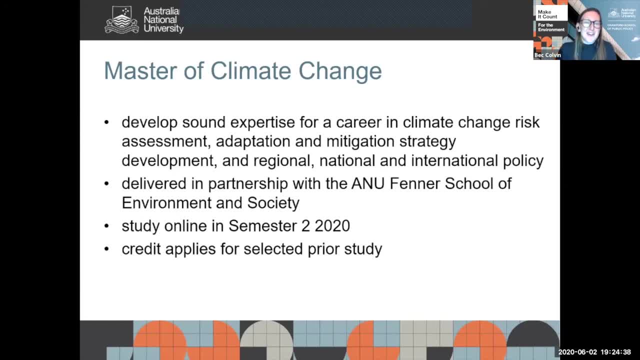 your new expertise in the area of climate change that is of most interest to you, And so you take these foundational courses and the climate change courses and your research project and a bit of research methods in the lead up to that. But you've also got a fair bit of latitude. 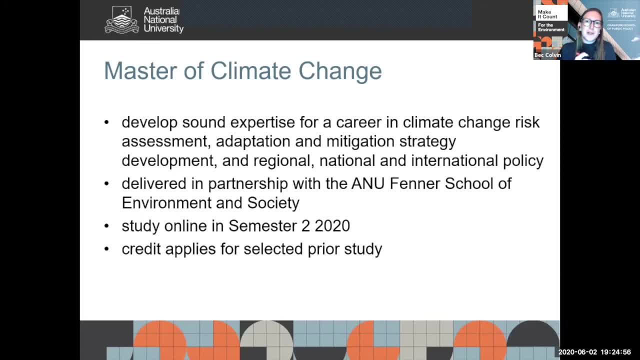 with electives as well, So you can tailor the program to suit a specialization, not a formal specialization, but if you are interested more so in the policy aspect or the social dimensions or climate science or the impacts, So we also will approve for other courses. 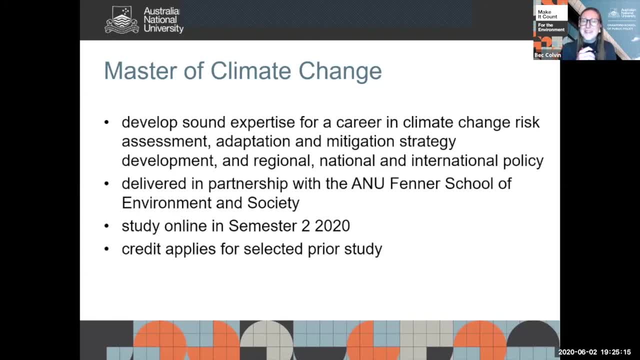 If you look at our elective list it's quite broad, But we also can make it broader than that if you find other courses from across the university that you can make a case for being relevant to your program. So, similarly to Sangro's comments about the Master, 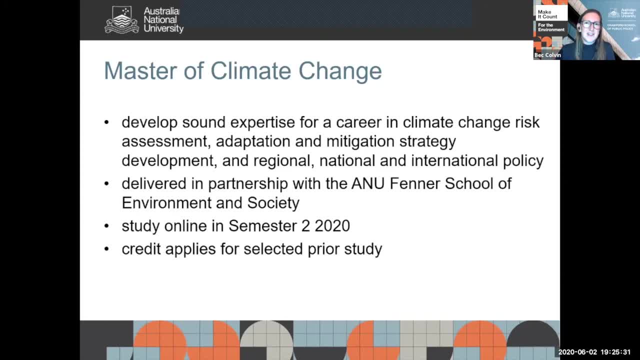 of Environmental Management and Development. this is a research-led course, So some of the teaching staff that you'll come into contact with are me. So I'm a social scientist and I'm interested in climate, energy, environmental policy and, in particular, social conflict and the role of identity. 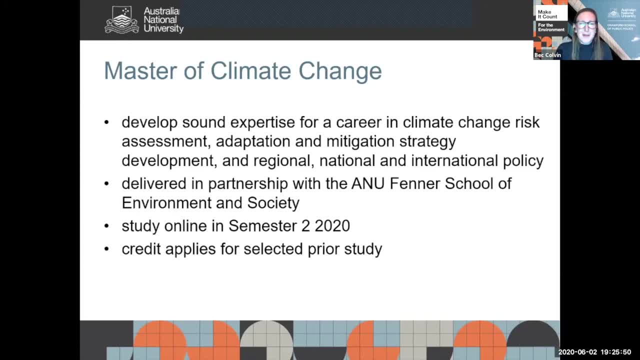 around these issues. I'm an intergovernmental panel on climate change contributing author. You'll also come across Professor Jamie Piddock. He's the other academic co-convener at the Fenner School. He's a professor at the University of Oxford. 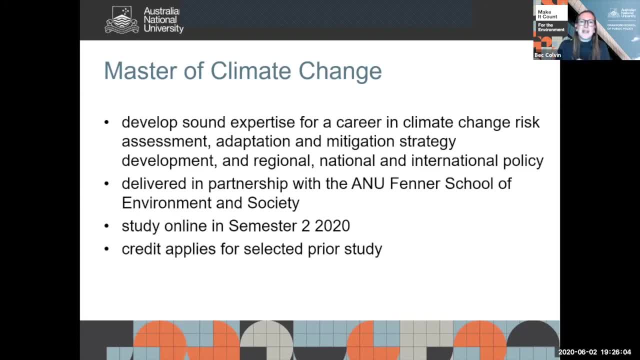 at the University of Oxford And he's a professor of environmental governance and adaptation and the nexus between climate change and water. And Professor Frank Jutso, who's here in the Crawford School, is a specialist in energy and climate policy and, in particular, the role of economic reform. 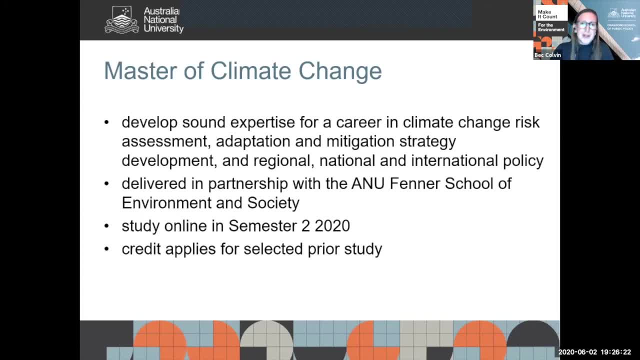 to deal with climate change. He's an IPCC lead author- And Dr Joelle Gerges, who's a climate scientist. She's the author of Sunburnt Country, seen in the bookstores a couple of years ago, And she's also an IPCC lead author. 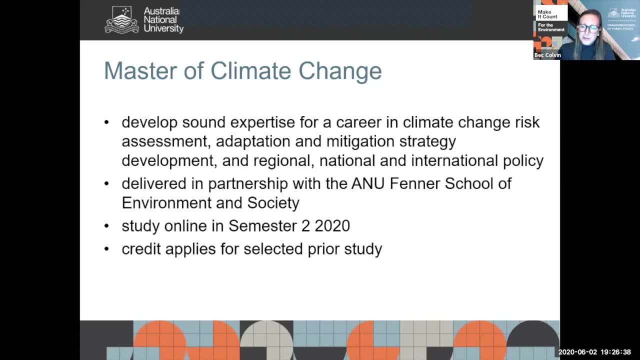 We also have at the ANU the ANU Climate Change Institute, which works across the university, And they focus on engaging our climate change researchers with the media and with the policy sector and with industry, And they host a whole suite of public events. 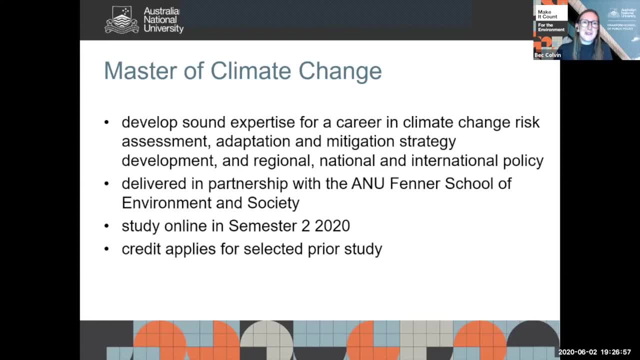 So the Climate Change Institute is another part of the university that you'll get embedded with It's standard, a two-year program, but you can get up to the equivalent of one-year course credit if you've got Cognate Study, And it's really fun. So it would be great to see you in this course.